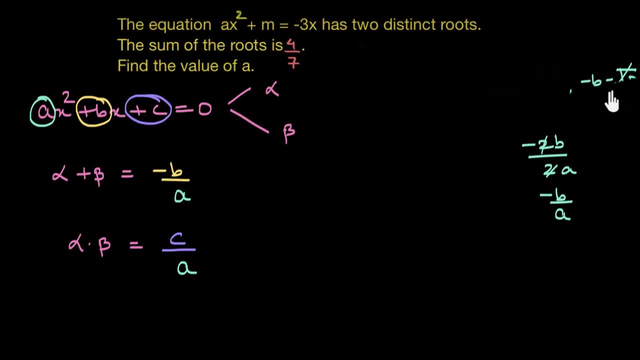 multiply them, you will get the product of the roots as c by a. So having said that, once we know what the relation between roots and the coefficients of a standard quadratic equation is, let's now try to solve this question. So in the question it is given that the 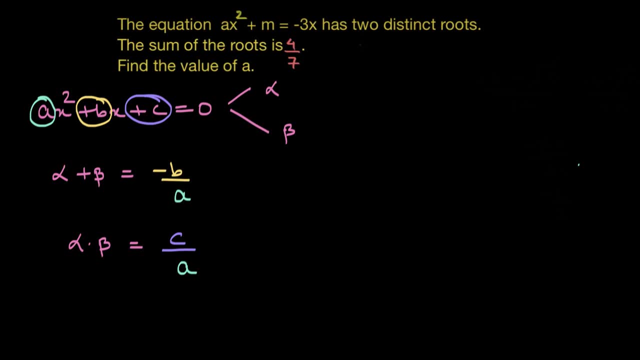 sum of the roots is 4 by 7, which means the value alpha plus beta is 4 by 7.. But make sure your quadratic equation is in standard form. In this case we have ax square plus m and this is equal to negative 3x. So we need all the terms of the quadratic equation to be able to solve this question. 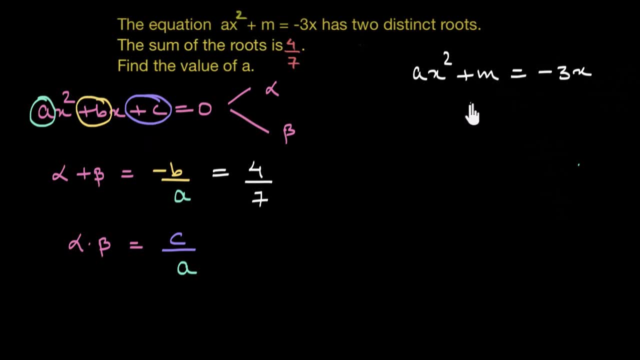 On one side of the equation. So in order to do that, we would add 3x on both the sides, So plus 3x and plus 3x. So this and this would cancel out. So we would be left with ax square plus 3x plus m. 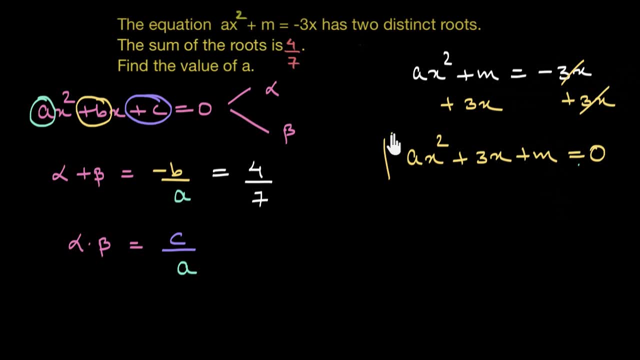 and this is equal to 0.. So now our quadratic equation is in standard form. So for this quadratic equation the sum of the roots would be given as negative of coefficient of x, that is, negative of 3 divided by coefficient of x square, that is a, So negative 3 upon a. This would be. 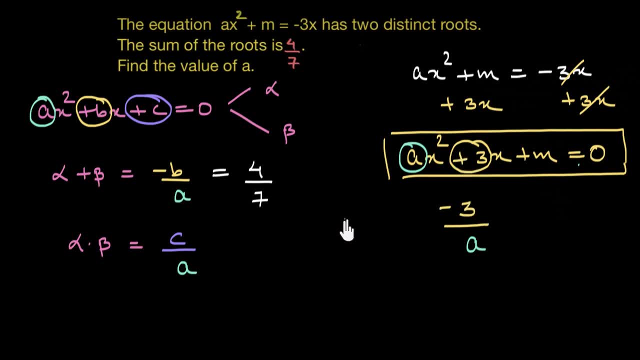 the sum of roots, alpha plus beta. But sum of the roots is given as 4 by 7, which means 4 by 7 is equal to negative 3 by a. Now, on multiplying both sides with a, on multiplying both sides with the reciprocal of 4 by 7, that is 7 by 4.. 7 by 4. 4 by 7 would cancel out 7 by 4 and we would be left. 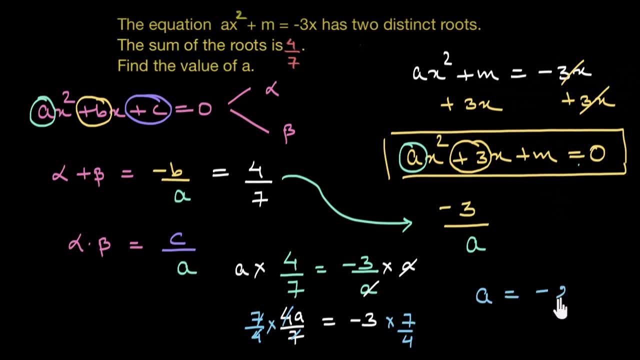 with a equals to negative. 7. 3's are 21 divided by 4.. So this is the value of a that we were looking for. The value of a that would satisfy the given equation, that is, the coefficient of x square would be equal to negative 21 divided by 4..